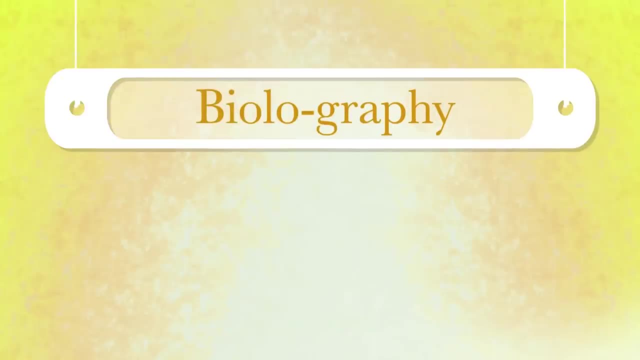 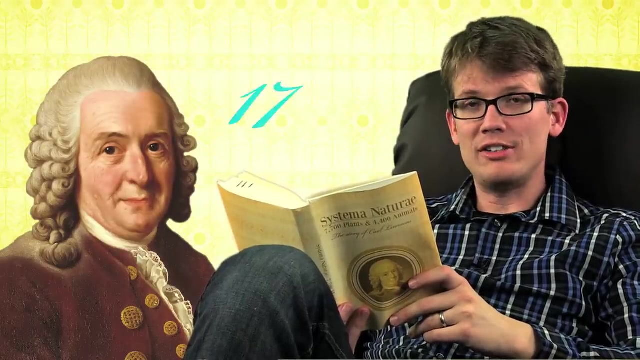 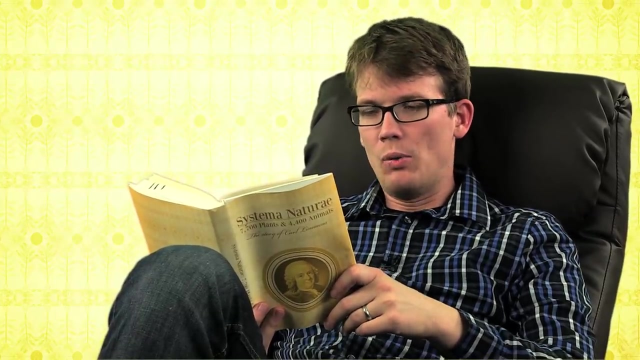 What's that? Do you smell a biography coming on? Carl Linnaeus was a Swede born in 1707,, and early in his career as a botanist he realized that the botanical nomenclature of 18th century Europe was well, just crap. For instance, in his day the formal name of a tomato plant was: Solanum caulea, enorme herbaceo, folis pinnatis incisus, racemus simplicibus. Linnaeus actually said Once: I shudder at the sight of most botanical names given by modern authorities. 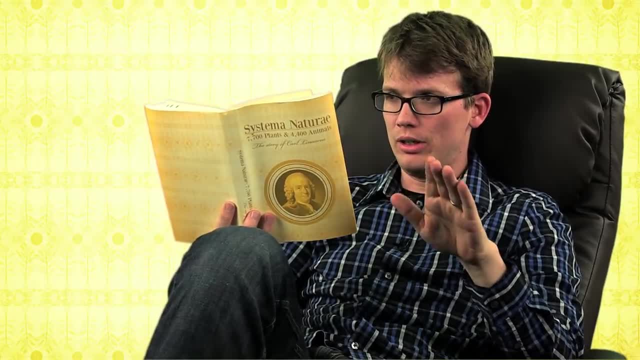 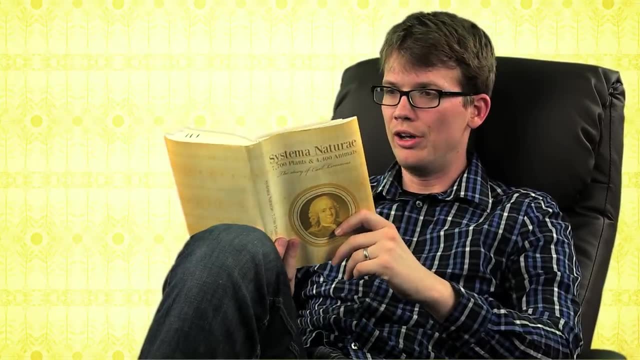 Not only did the slobbiness bother him, he saw a whole sugar storm blowing in because new plants were still being discovered in Europe. But that was nothing compared to the crazy stuff that was coming from the New World. Linnaeus saw that pretty soon. naming conventions were just going to collapse. 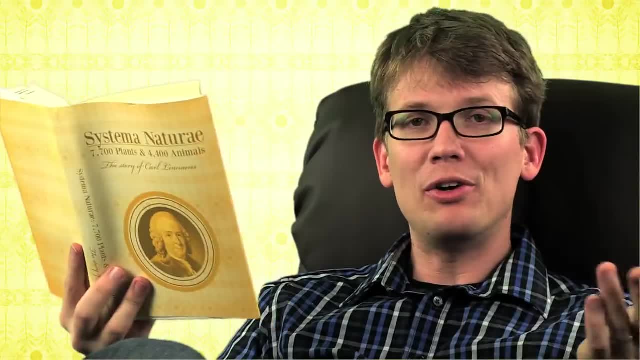 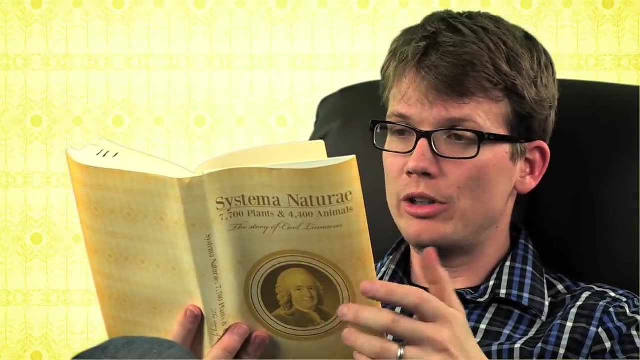 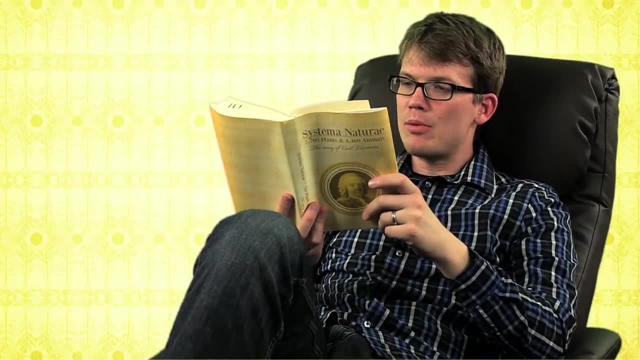 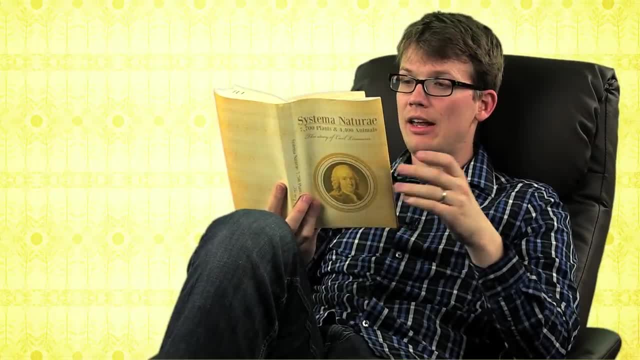 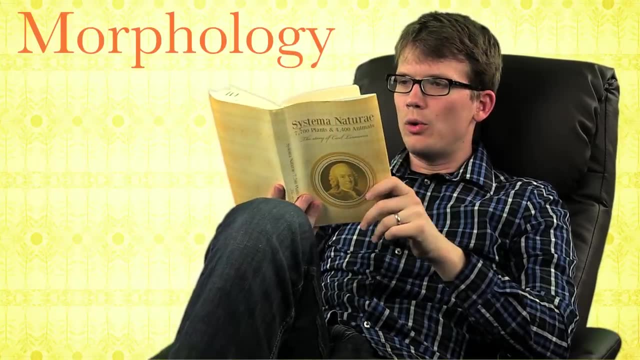 where he devoted himself to the study of nomenclature. He had his students go to places and bring back specimens for him to study and categorize. The method he eventually adopted was based on morphology or physical form and structure. This wasn't necessarily a new idea. 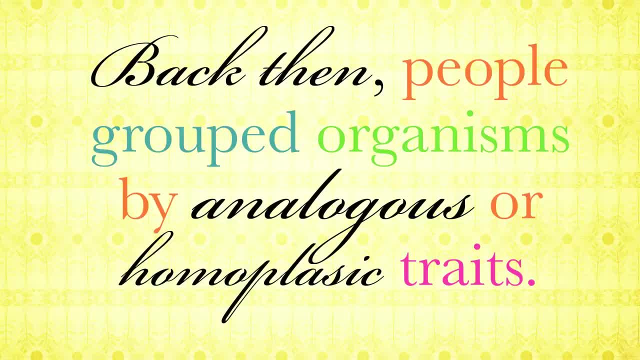 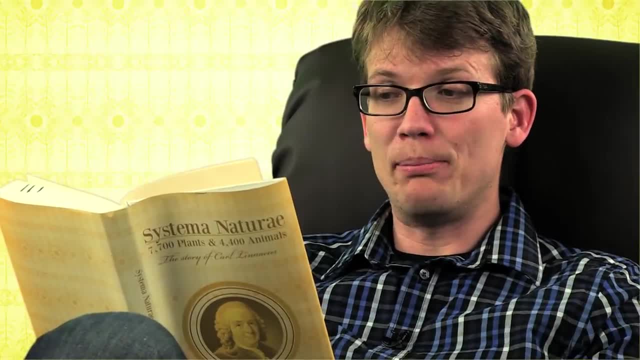 Back then, people grouped organisms by analogous or homoplastic traits, structures that appear similar but actually come from completely independent origins. By this definition, birds would be more closely related to butterflies than to reptiles, because both birds and butterflies can fly. 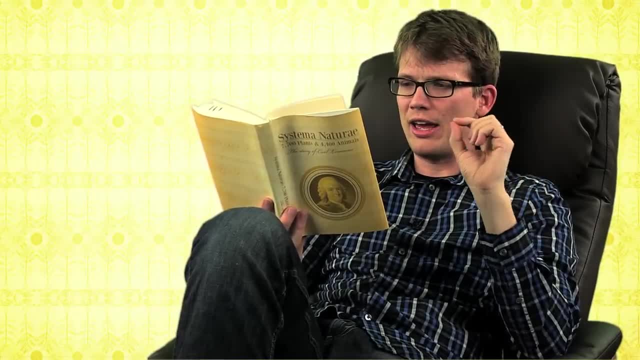 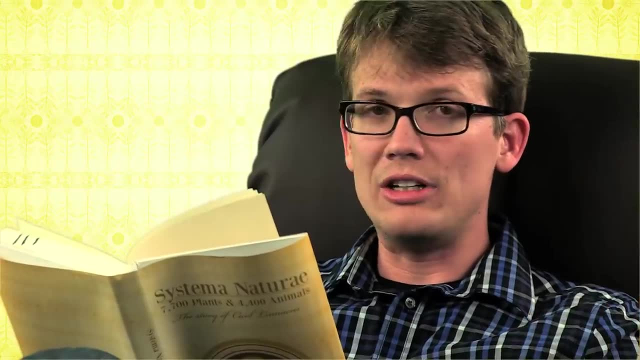 But Linnaeus had a good mind for this stuff and turned it to have a real knack for choosing actual homologous traits for his classification system, Traits that stem from a common evolutionary ancestor. Linnaeus, of course, didn't know jack about evolution. 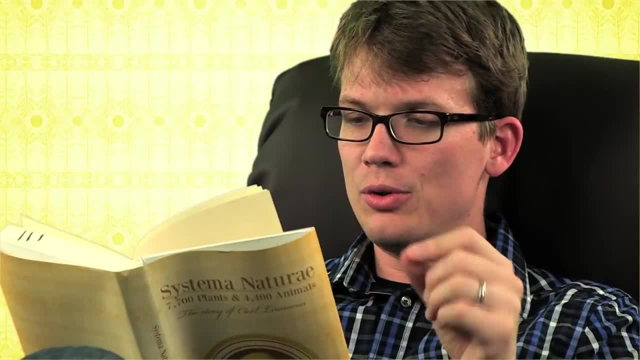 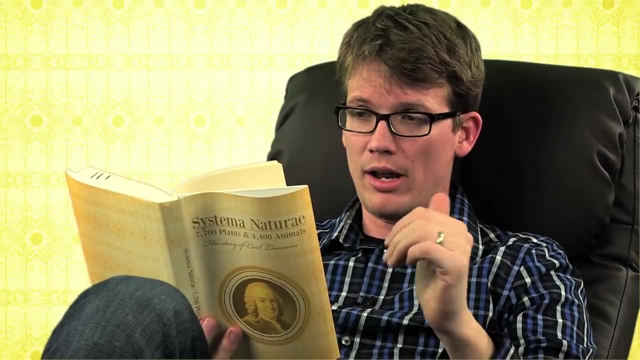 Darwin wouldn't come around for another hundred plus years, but he intuited that some traits were more important than others. For instance, he was struck by the fact that reproductive apparatus seemed to be a good way of classifying plants. He also caused a bit of a scandal by classifying class. For instance, he was struck by the fact that birds were more likely to produce milk from their nipples than females, Because apparently that was pretty racy stuff back then. In his lifetime, Linnaeus cataloged roughly 7,700 plants and 4,400 animals. 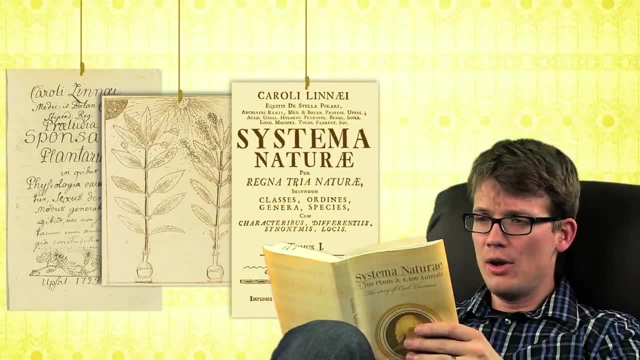 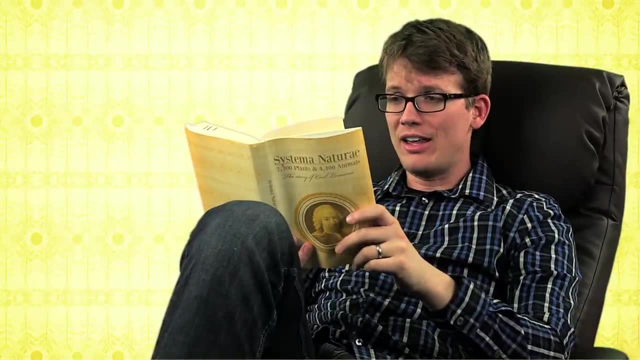 He published his classifications in a catalogue called Systema Naturae which, by the time he wrote its 12th edition, was 2,300 pages long. In the meantime, Linnaeus actually adopted a personal motto: God created, Linnaeus organized. 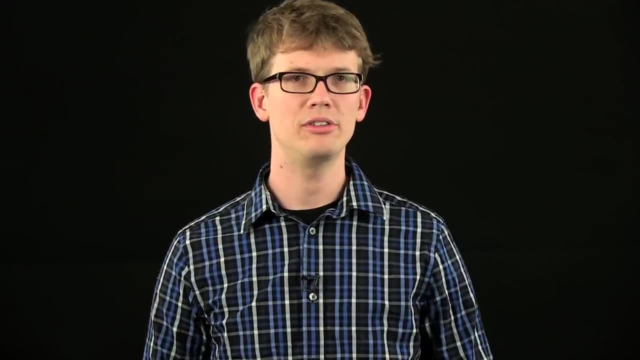 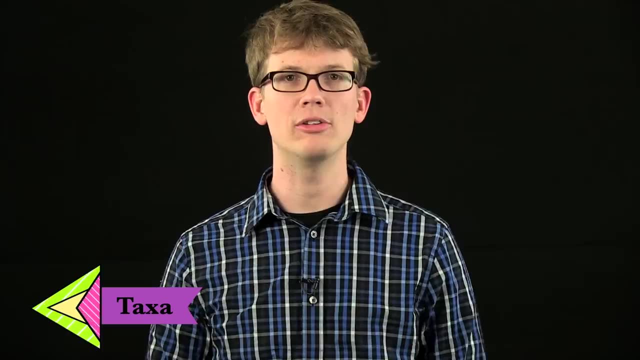 Although taxonomy has come a long way, A long way- since Linnaeus, we still use a bunch of the conventions that he invented. For instance, we still arrange things into taxa or groups of organisms, and we still use the same taxa as Linnaeus. 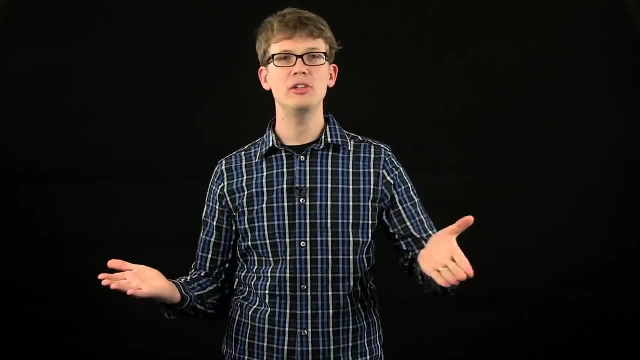 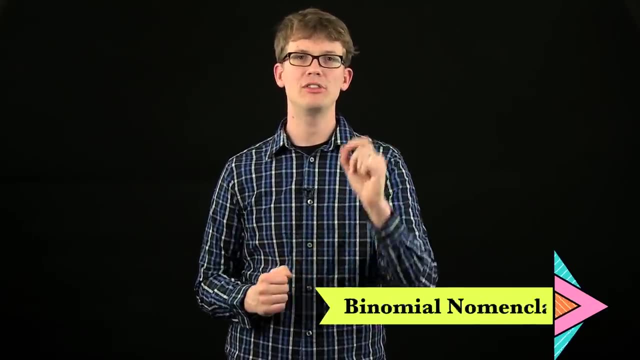 Kingdom file and class order, family, genus and species. We also still use Linnaeus' convention of binomial nomenclature, using a unique two-part name for every species: The genus and its species name In Latin or sort of Latin-ish. This practice actually started back in the middle ages, when educated people were expected to know Latin. We don't use Latin now, but we know a lot more about evolution which Linnaeus didn't, And we have technologies like genetic testing to classify relationships between organisms. 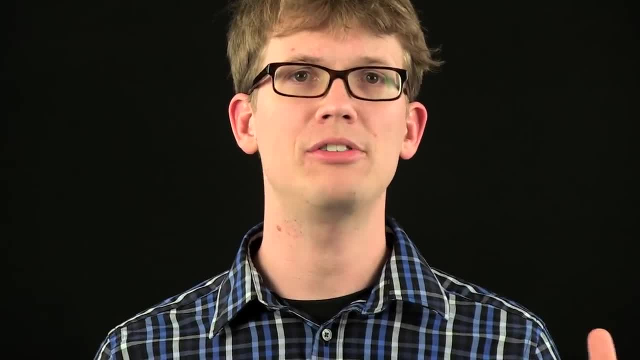 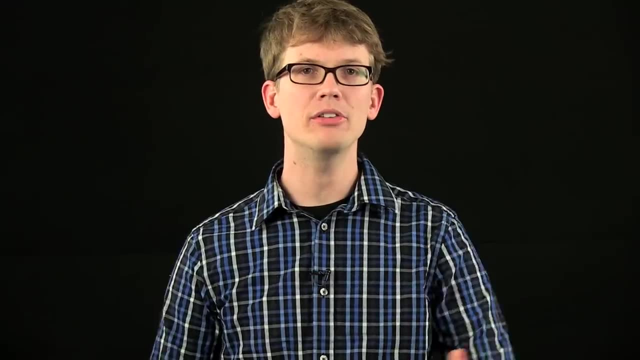 And yet we still use Linnaeus' morphology-based system because genetic evidence generally agrees with classifications that are made based on structure and form. However, because there was a lot of life that Linnaeus had no idea about, we had to stick. 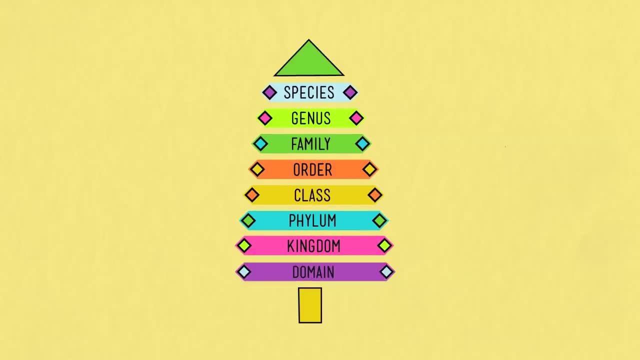 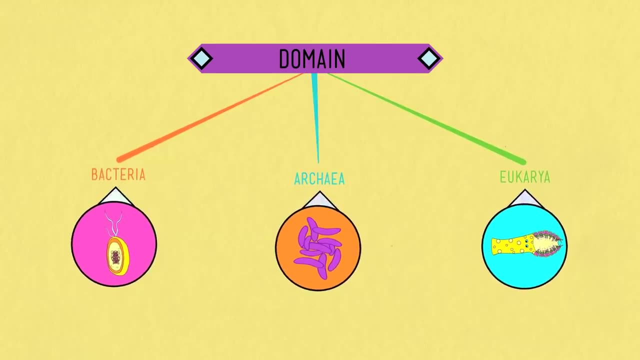 a new taxa above Linnaeus' kingdom. We call it Domain And it's as broad as you can get. The domains are Bacteria, Archaea and Eukarya. The bacteria in the Archaea are prokaryotes, meaning that their genetic material goes commando. 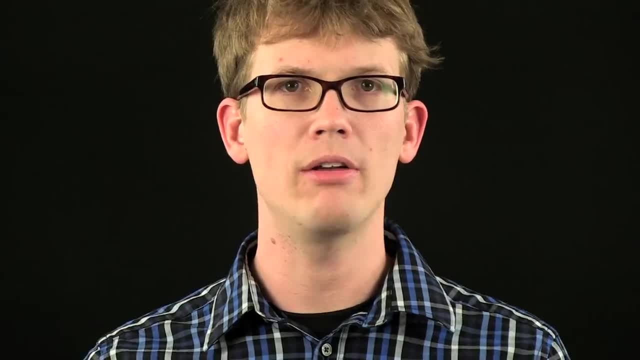 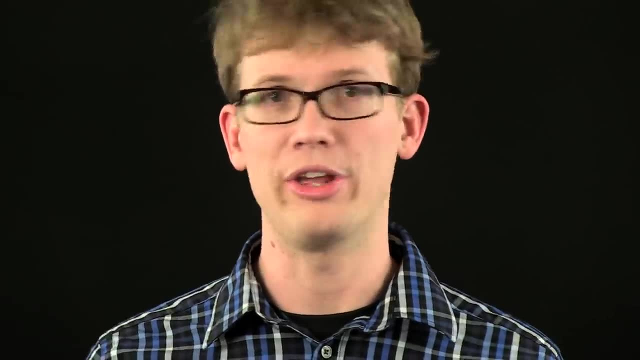 with no nucleus to enclose it, while the Eukarya make up all of the life forms with a nucleus and include pretty much all of the life that you think of as life and quite a lot of the life that you don't think about at all. 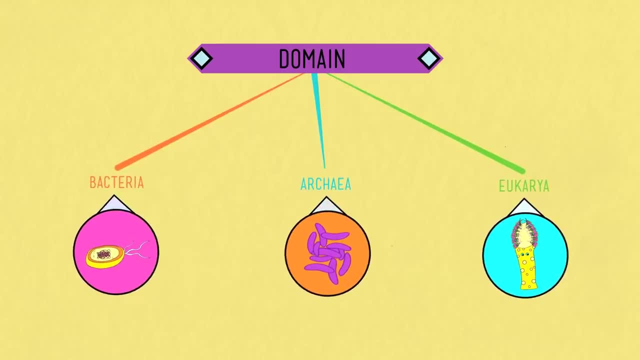 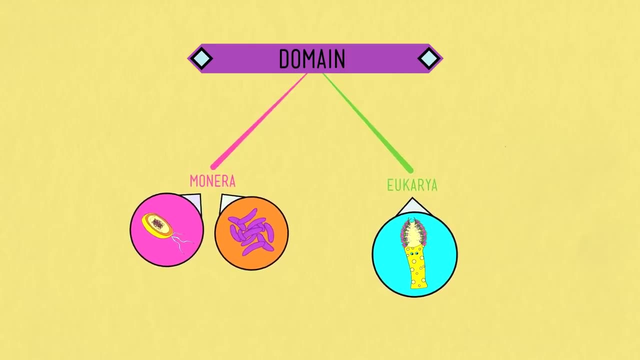 It might seem like, since all macroscopic life only gets one domain, it's kind of silly to give prokaryotes two, And for a long time we didn't In the different domains. they hung out together in a single domain called Monera. But it later became clear that Bacteria, which live pretty much everywhere on Earth, including inside of you and deep in the Earth's crust, and Archaea, which are even more hardy than Bacteria, have distinct evolutionary histories, Archaea being more closely related to Eukaryotes and, yes, thus me and you. they have totally. 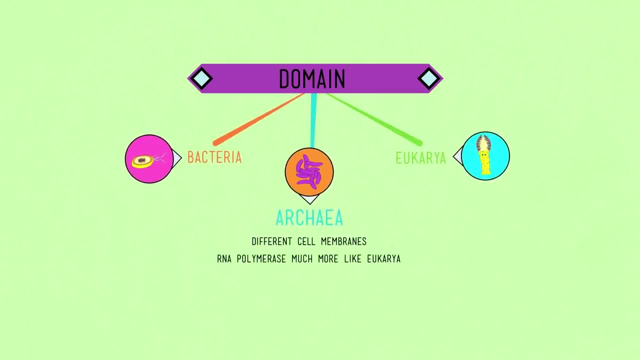 different cell membranes and the enzymes that they use to make RNA. their RNA polymerase is much more like ours Under the domain Eukarya, which is by far the most interesting domain in the world. Archaea is one of the most interesting domains in the world. 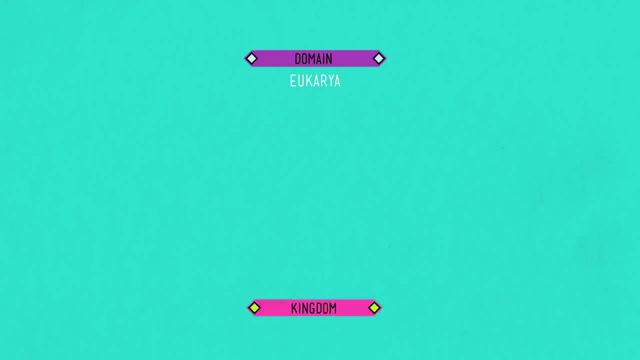 Archaea is one of the most interesting domains in the world, And in the most interesting and even occasionally adorable domain we have kingdoms Protista, Fungi, Plantae and Animalia. Now scientists have settled on these four for now. 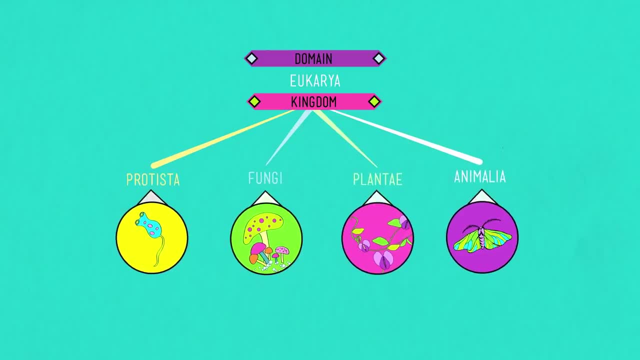 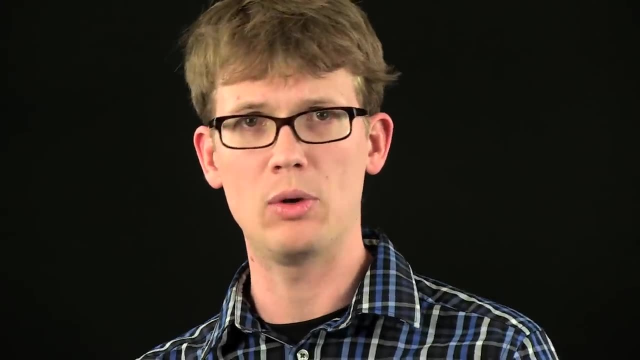 But these are categories that are a human creation. But there are good reasons for that human creation. The unscientific truth is that we looked at life and divided it up based on what we saw, So we were like: well, protists are single-celled organisms, so they're very different from 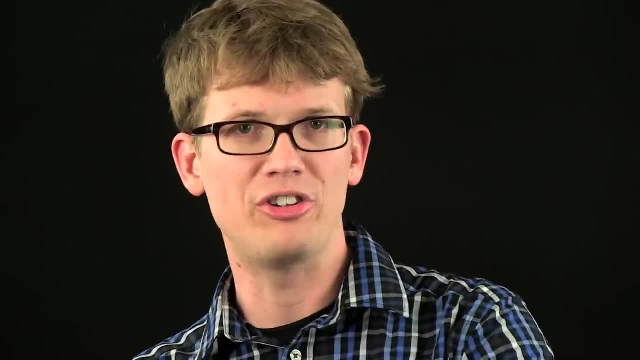 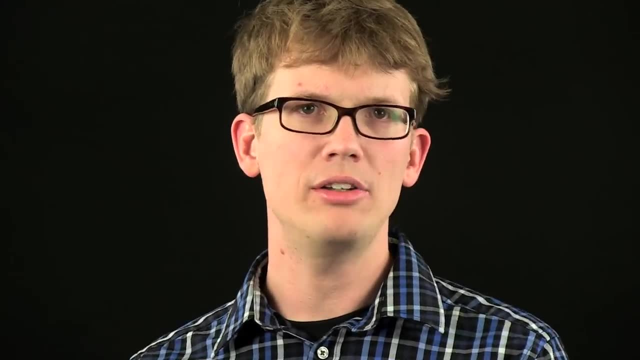 the rest of the domain, And plants get their energy from the sun, and fungi look and act very different from plants and animals, And you know, we already know what animals are. so they have to get their own kingdom And though scientists are sometimes loath to admit it, that system of just looking and 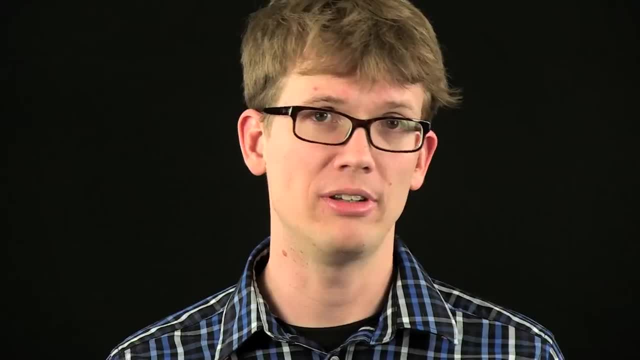 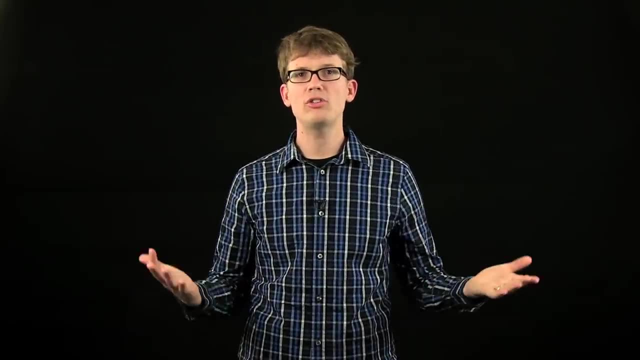 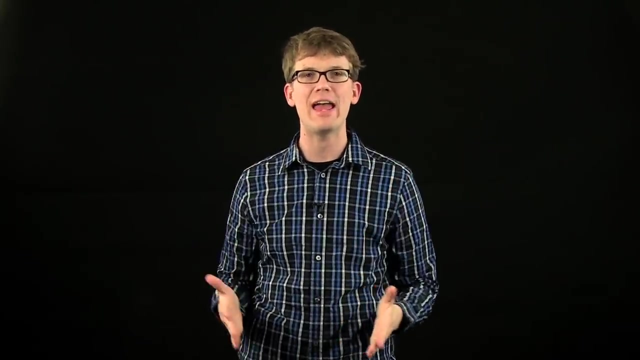 dividing things up actually worked pretty well for us- Not perfectly, but pretty well. But there's a reason why this worked so well: Evolutionarily. there are actual categories. Each of these kingdoms is a huge branch in the tree of life. At each branch, an evolutionary change occurred that was so massively helpful that it spawned. 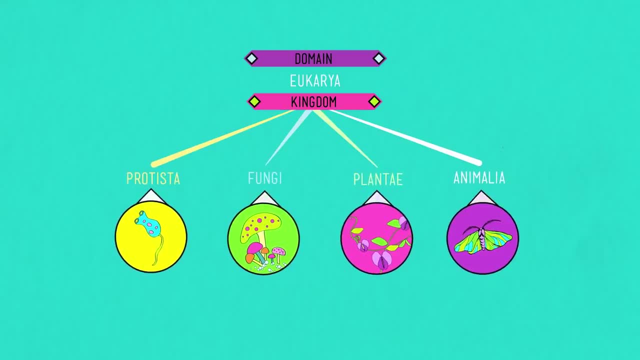 a vast diversity of descendants. Plants, or plantae, are the autotrophs of the domain Eukarya, Autotrophs meaning that they can feed themselves through photosynthesis. of course, There's cellulose-based cell walls and chloroplasts, giving them a distinct difference from all. 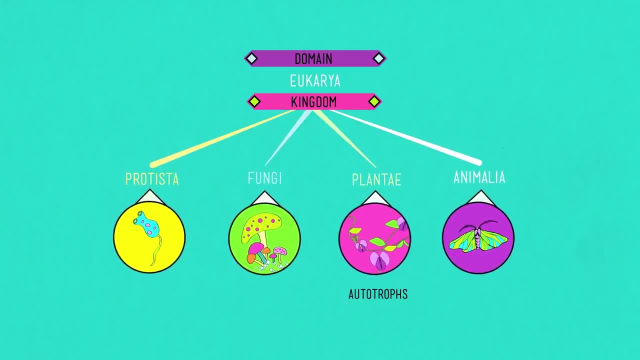 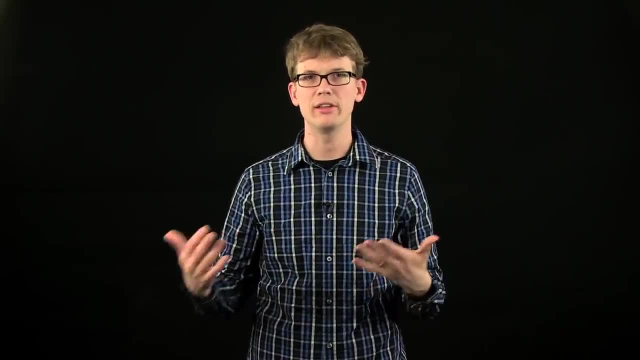 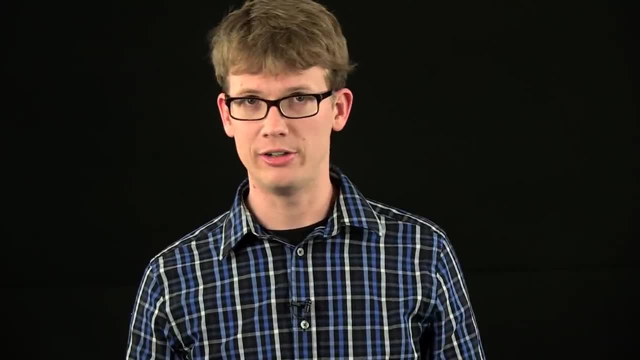 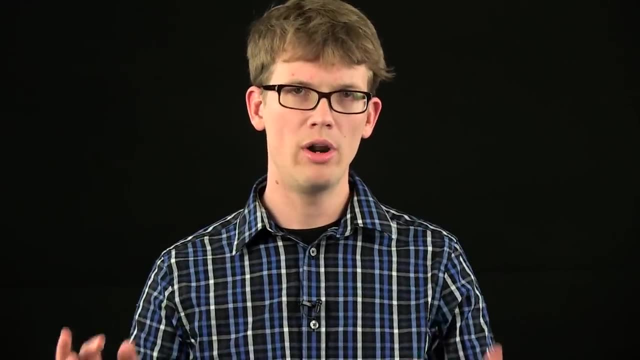 be evolutionarily related to each other. Scientists are still trying to figure it out. Some are plant-like, like algae, Some are more animal-like, like amoebas, And some are fungus-like, like slime molds. Protists are one of those gray areas I was telling you about, so don't be surprised. 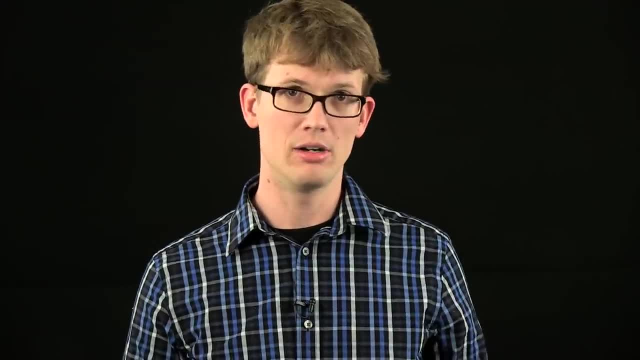 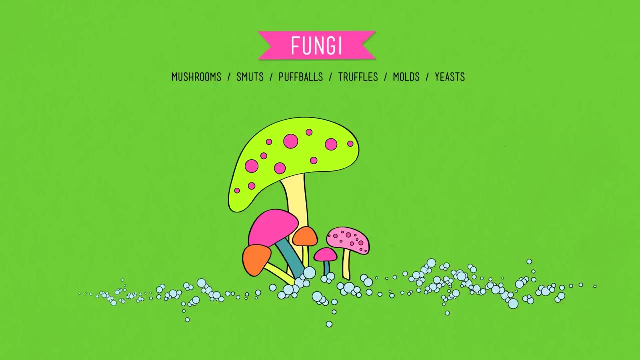 if, by the time you're teaching this to your biology students, there are more than four kingdoms in Eukarya Which are, you know, the funguses? They include mushrooms and smuts and puffballs and truffles and molds and yeasts. 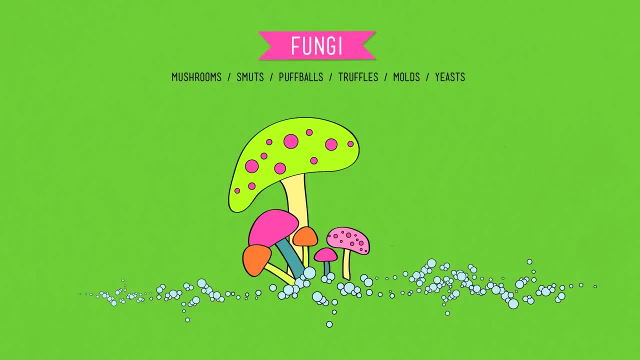 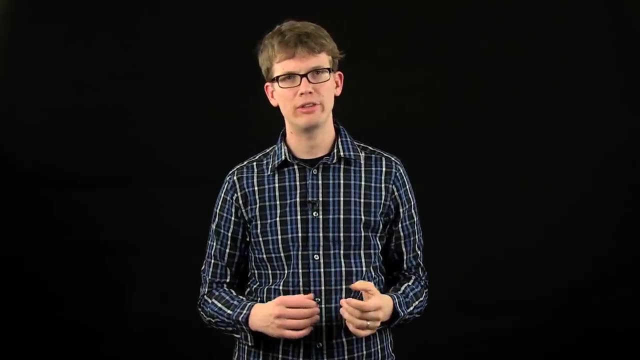 And they're pretty cool because they have cell walls like plants. but instead of being made of cellulose, they're made of another carbohydrate called chitin, which is also what the beak of a giant squid is made of, or the exoskeleton of a beetle. Because fungi are heterotrophs, like animals. they have these sort of digestive enzymes that break down their food and get reabsorbed, But they can't move, so they don't require a stomach for digestion, they just grow on top of it. 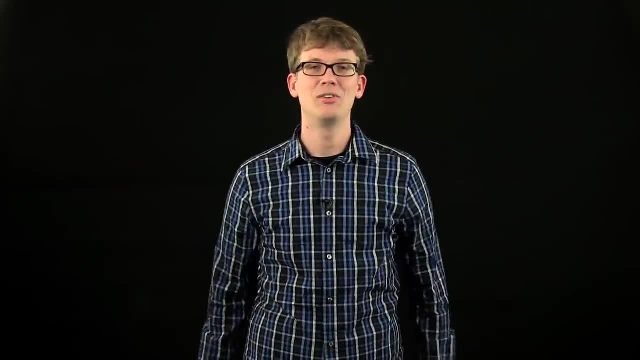 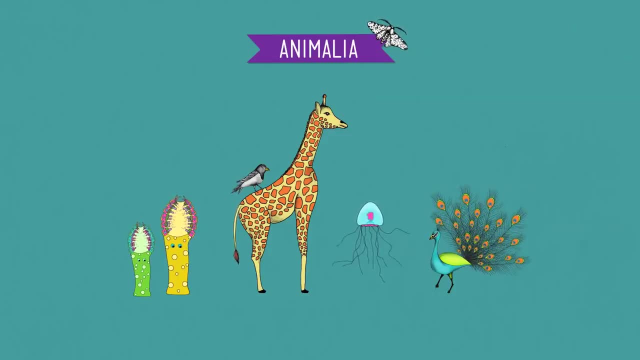 On top of whatever it is they're digesting, And digest it right where it is, which is super convenient. And finally, we have kingdom animalia, which is the lovely kingdom that we find ourselves and 100% of adorable organisms in. 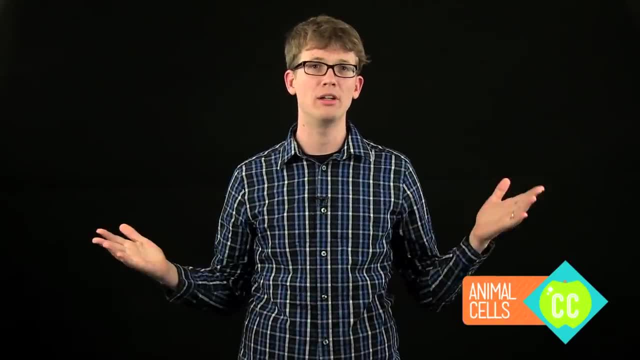 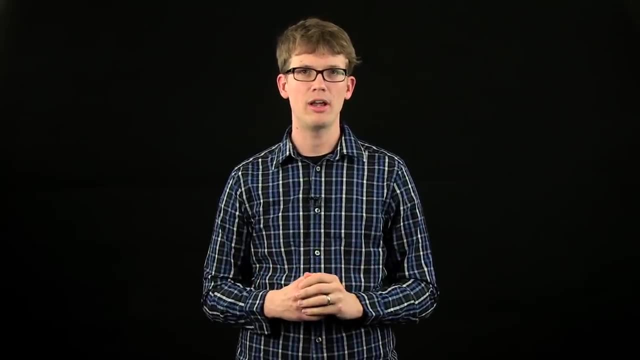 Animals are multicellular, always We are heterotrophic, so we spend a lot of time hunting down food because we can't make it ourselves. And almost all of us can move, at least during some stage of our life cycle, And most of us develop either two or three germ layers during embryonic development. 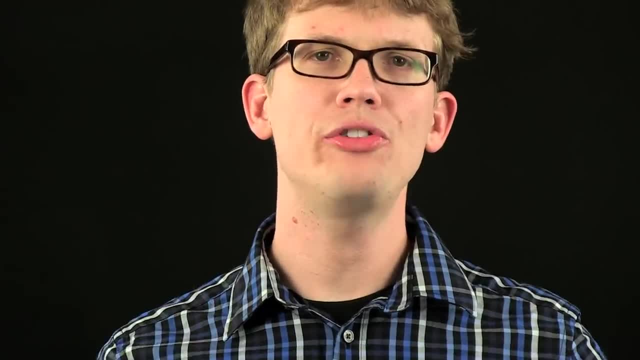 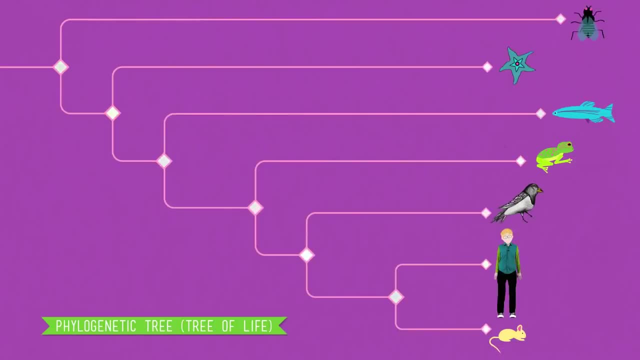 Wait for it, Unless you're a sponge. So, like I said, we use this taxonomic system to describe the common ancestry and evolutionary history of an organism. Looking at the phylogenetic tree, you can tell that humans are more closely related to mice than we are to fish and more closely related to fish than we are to fruit flies. 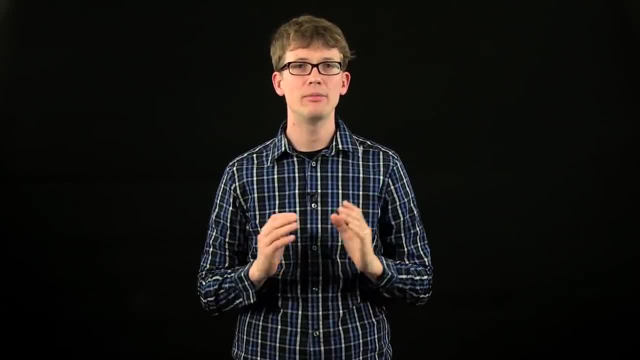 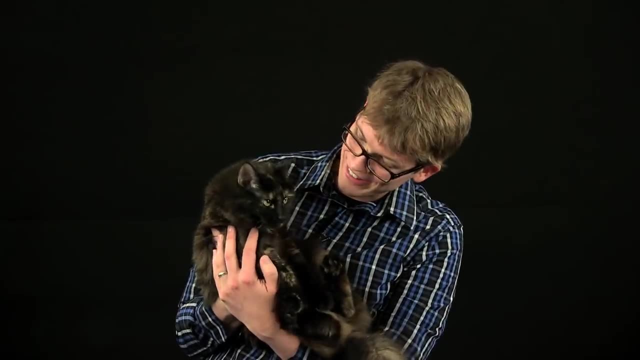 So how about we pick an organism and we follow it all the way through the taxa from kingdom to species just to see how it works? I know Let's pick this kitty Because I know she'd like it, Right cat? 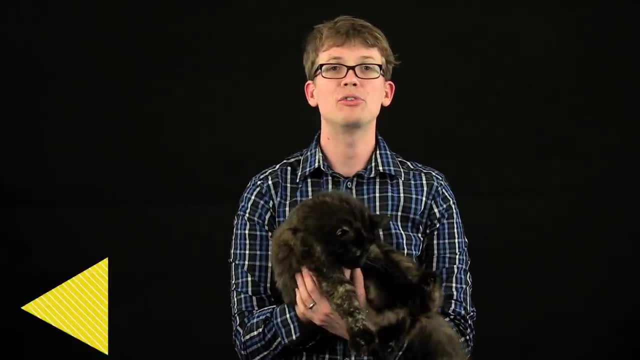 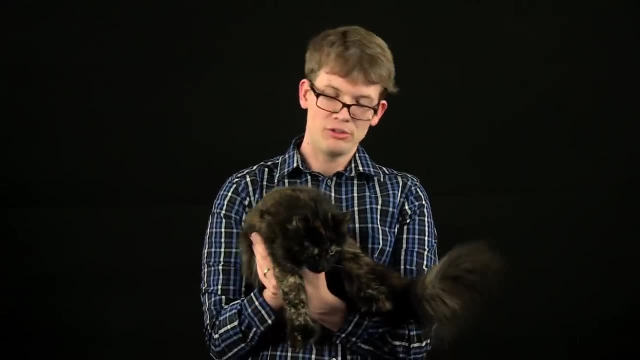 So kitties have cells that have nuclei and membrane-surrounded organelles and they're multicellular and heterotrophic and have three germ layers of cells when they're embryos so they're in the kingdom Animalia And they have a spinal cord running down their backs, protected by vertebrae and discs in. 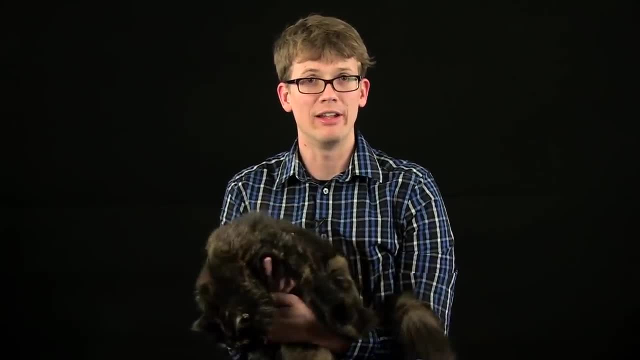 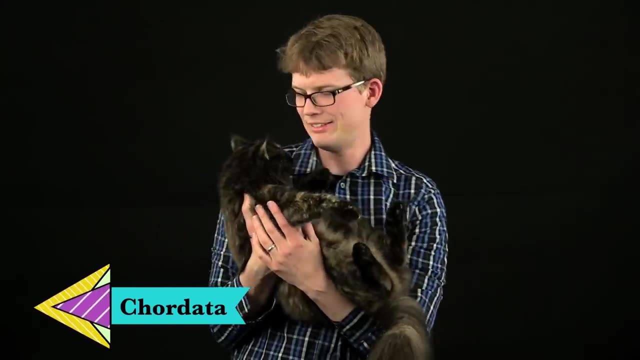 between them And they have a tail that doesn't have a butthole at the end of it like a worm, which I'm really glad about, And that puts her in the phylum Chordata. Kitty clearly does not like this, so I'm going to put her down now. 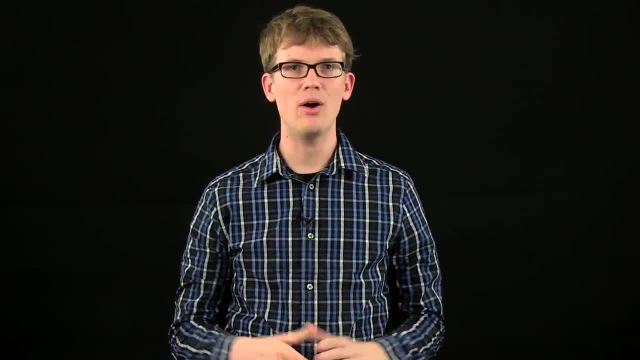 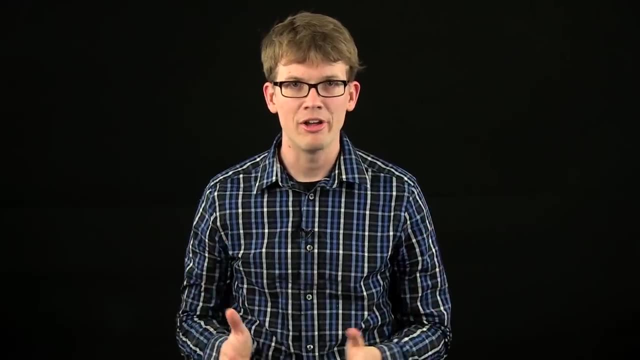 And the kitty lactates. It gives birth to young like a cow instead of laying eggs like a chicken, And they have fur and three special tiny bones in their ears that only mammals have, So they're in the class Mammalia. 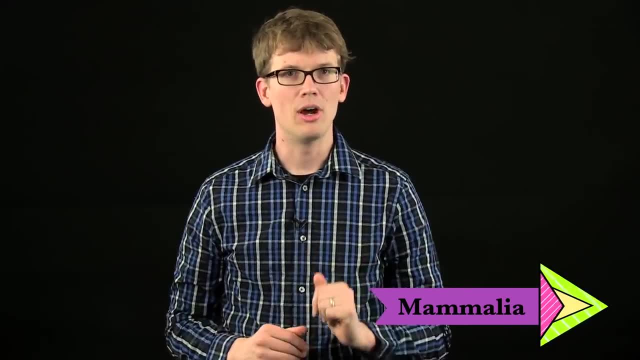 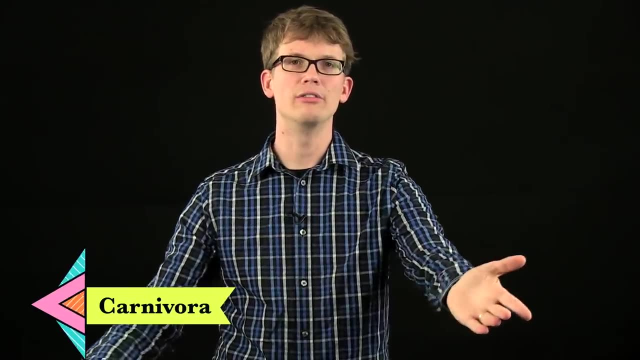 So she's more closely related to cow than to chicken, Good to know. And like a bunch of other placental mammals that eat meat, like weasels, the mustelids and dogs, the canines kitties are in the order Carnivora. And they're in the cat family Felidae, whose members have lithe bodies and roundish heads and, except for cheetahs, retractable claws, And they're littler than tigers and panthers, which puts them in the genus Felis. 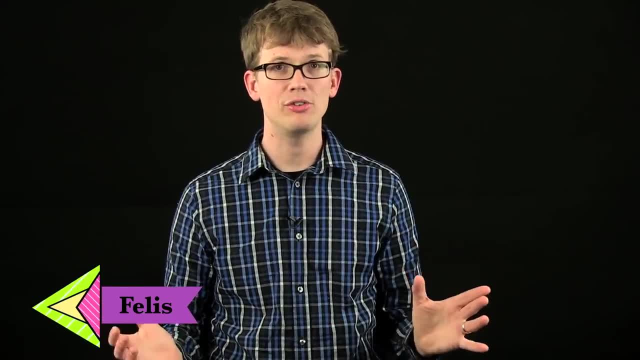 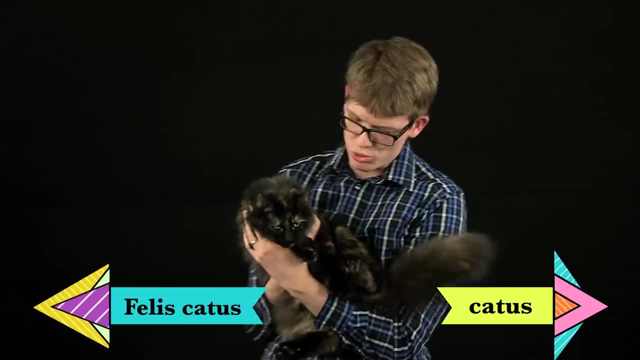 And then, at the level of the species, the descriptions get pretty dang detailed. So let's just say that you know what a cat is. So the species name is Catus, And look at that: Felis Catus. Aw kitty, I could have that whole thing cross-stitched onto a pillow for you to sleep on.